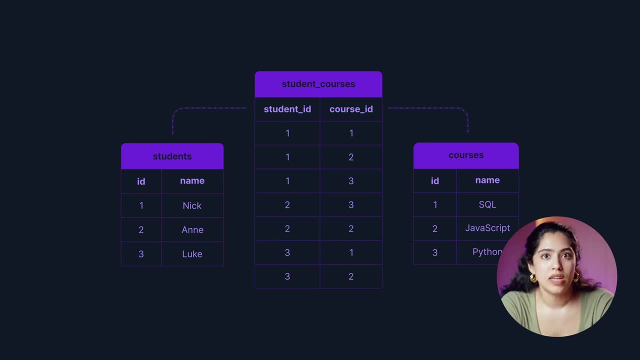 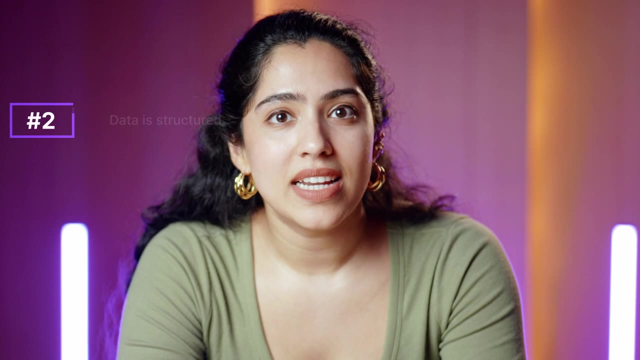 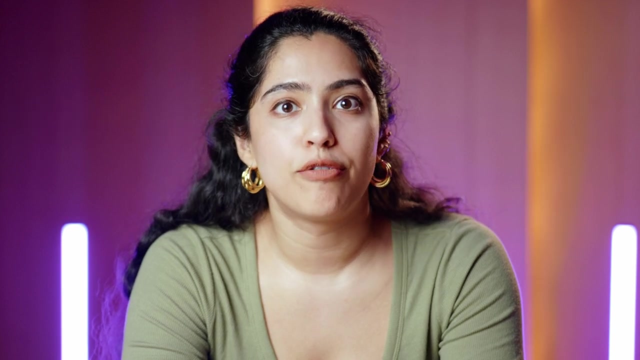 relationships between data among multiple tables. Table relationships are really important for effectively organizing and structuring a lot of different data. Second, the data is well structured and the room for potential error is therefore reduced. This is because SQL schemas require the data model and format of the data to be known before storing. 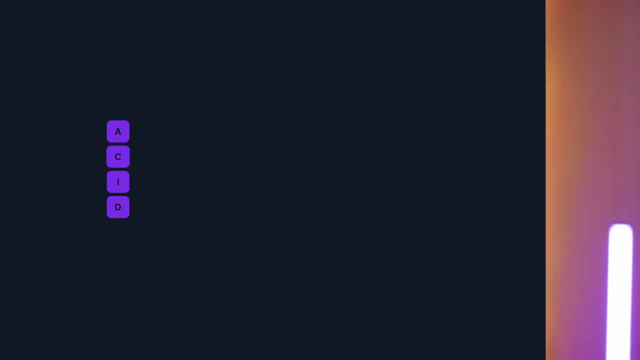 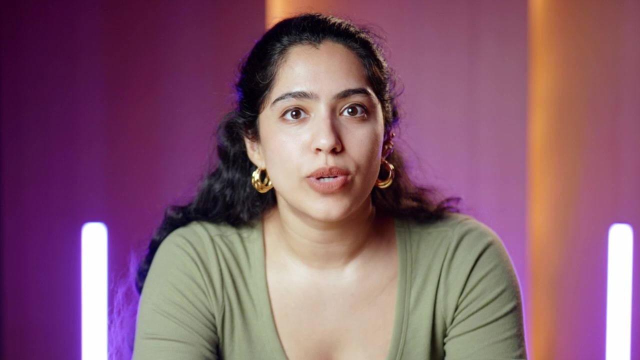 anything. Third, SQL databases are ACID compliant. This means that transactions are atomic, consistent, isolated and durable. SQL transactions are groups of statements that are executed atomically. This means that the data is well structured and the room for potential error is therefore reduced. 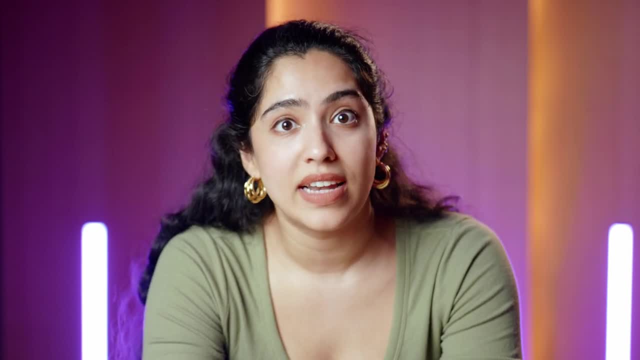 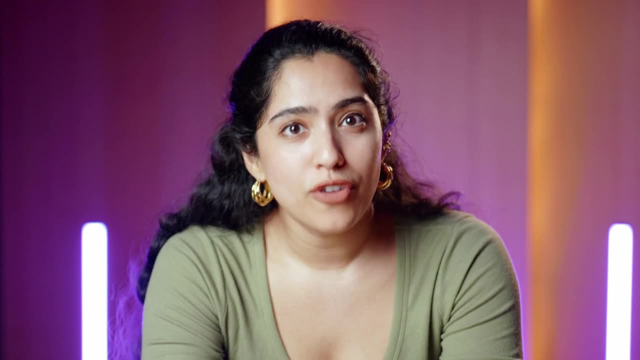 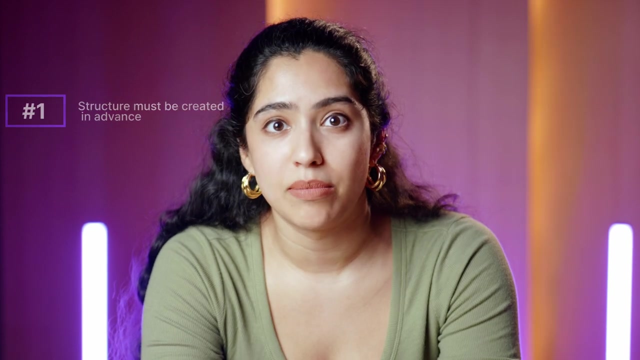 either all executed or not executed at all if any statement in the group fails. With all these strengths, SQL sounds great. so what are its weaknesses? Well, first, structured data might mean fewer errors, but it also means that columns and tables have to be created ahead of time, So SQL databases take more time to set up. 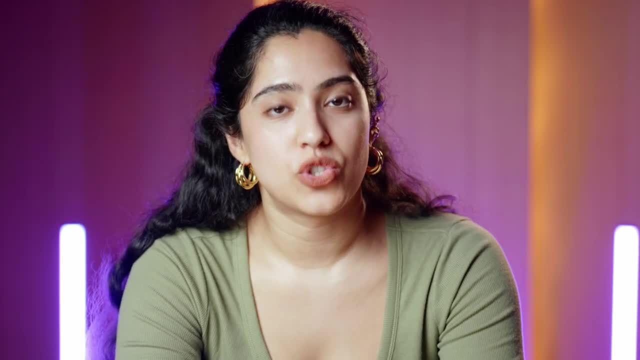 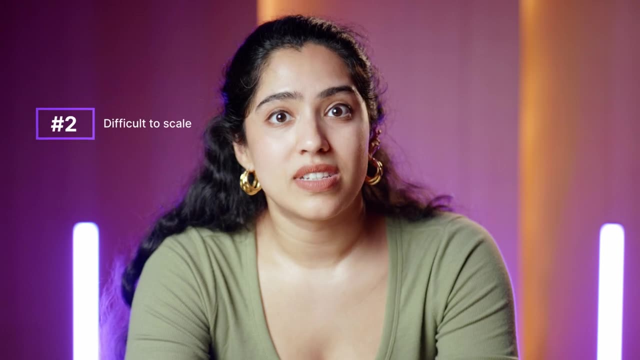 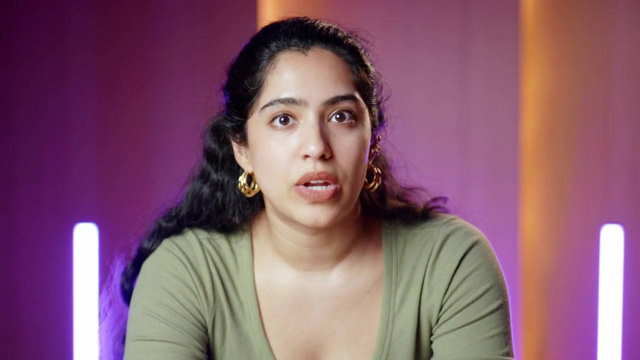 compared to NoSQL databases. They're also not effective for storing and querying unstructured data where the format is unknown. Second, SQL databases are highly structured and the room for SQL databases is limited. SQL databases are difficult to scale horizontally because of their relational nature. For read-heavy systems, it's straightforward to provision multiple read-only. 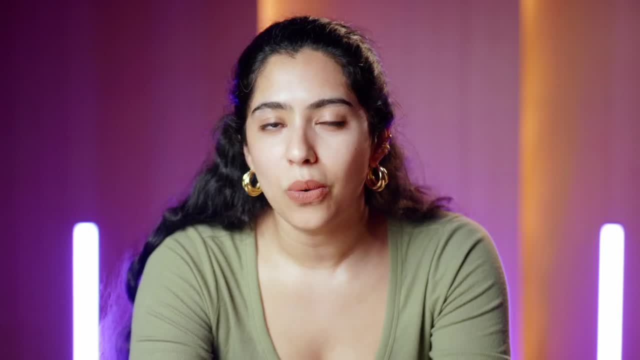 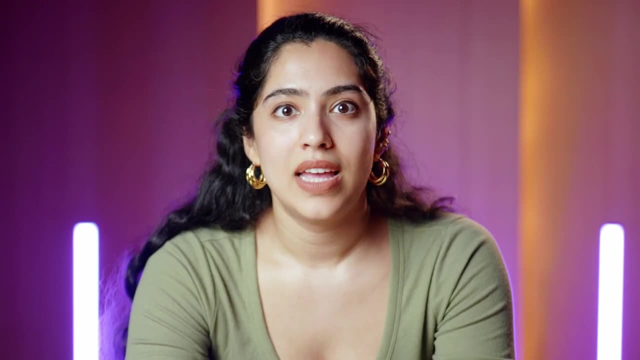 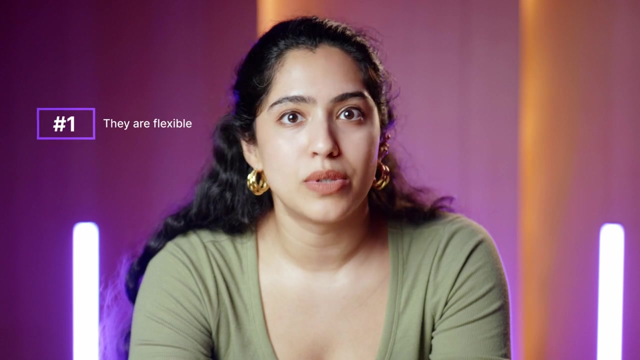 replicas. but for write-heavy systems, usually the only option is to vertically scale the database up, which is generally more expensive than provisioning additional servers. Now let's talk about the benefits of NoSQL databases. First, NoSQL databases are more flexible and simpler to set up because they do not support table-related 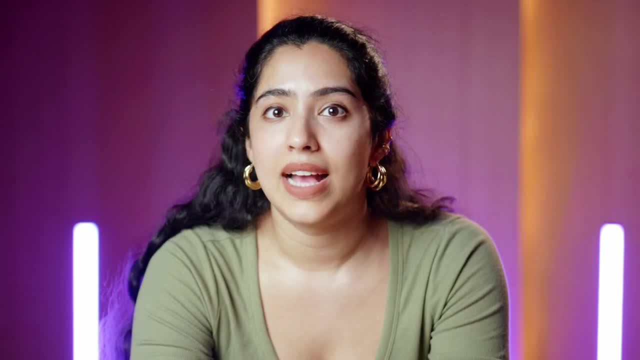 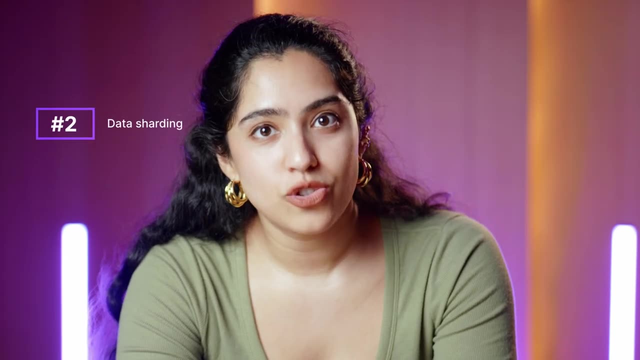 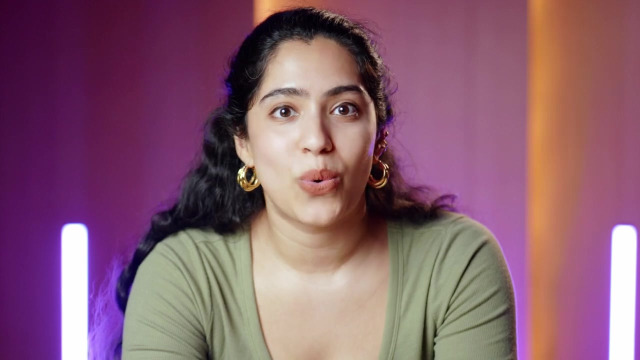 relationships and data is usually stored in documents or as key-value pairs. They're a better choice for storing unstructured data. Second, because they're better at handling unstructured data, they can also shard this data across different data stores, allowing for distributed databases. This makes horizontal scaling much easier and very large amounts of 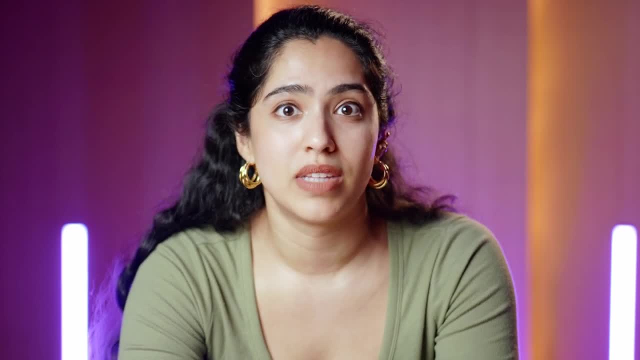 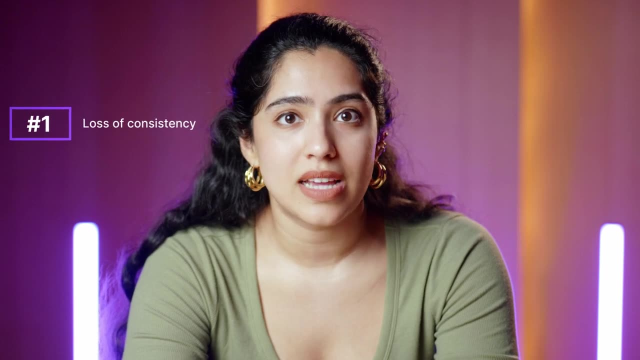 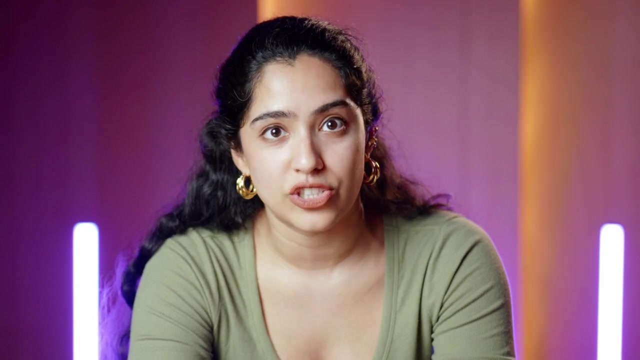 data can be stored without having to purchase a single expensive server. But NoSQL databases also have their weaknesses. NoSQL databases are typically designed for distributed use cases, and write-heavy systems can be supported by having multiple write shards for the same data partition. This is called peer-to-peer replication. However, the trade-off is a loss of strong consistency. 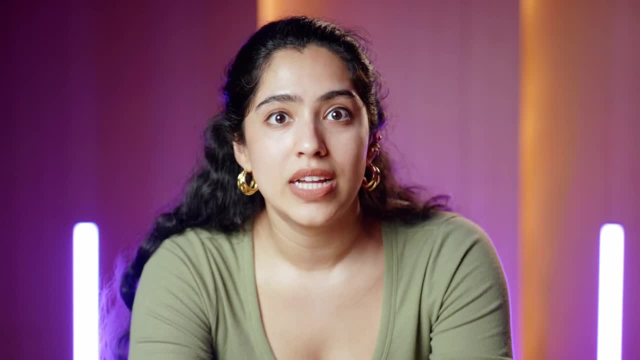 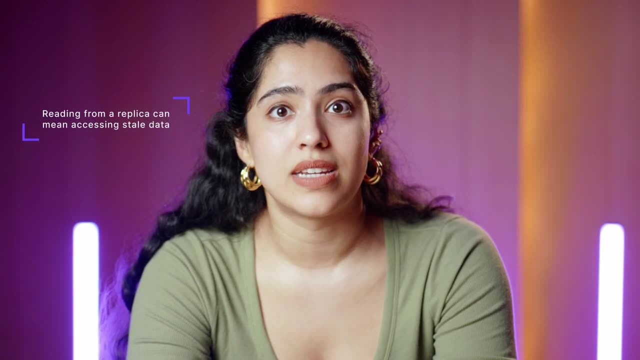 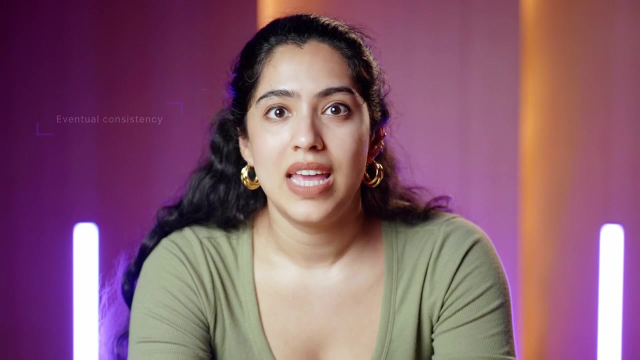 After a write to a shard in a distributed NoSQL cluster, there's a small delay before that update can be propagated to other replicas. During this time, reading from a replica can result in accessing stale data. This weakness of the data being up to date is called eventual consistency. Eventual consistency isn't exactly a fault of just. 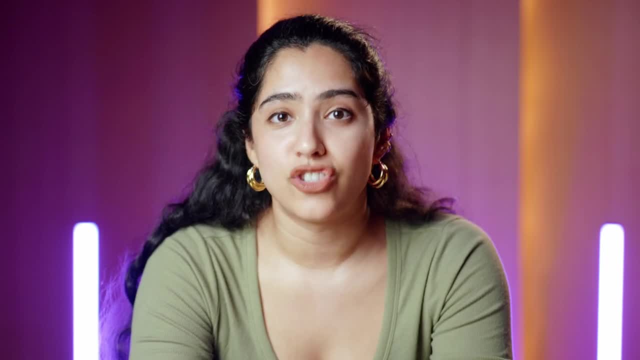 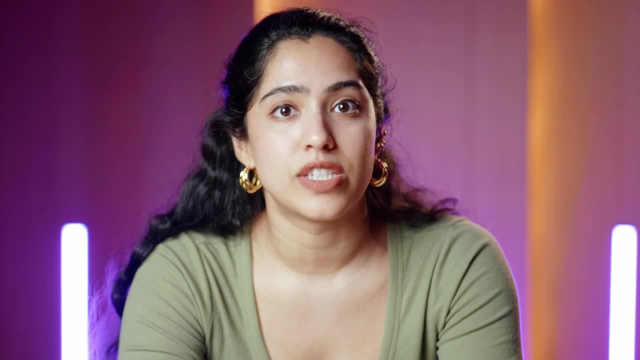 NoSQL databases, but of distributed databases in general. A single shard NoSQL database can be strongly consistent, but to fully take advantage of the scalability benefits of NoSQL, the database should really be set up as a distributed cluster. And that's it for today's video on databases.